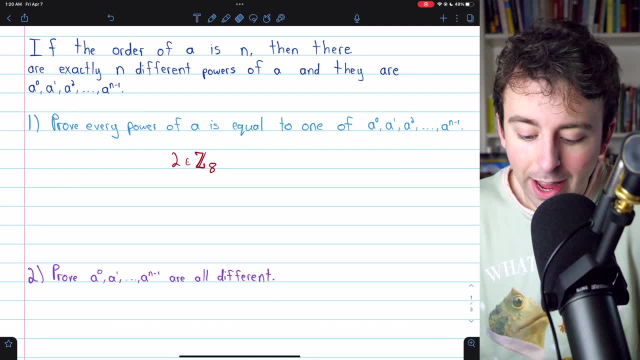 example to make sure we understand what this result is saying. Consider two. 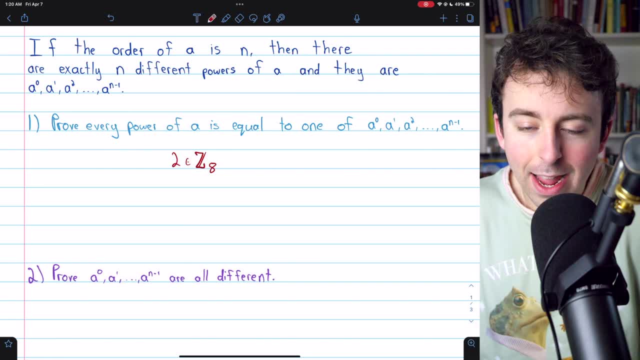 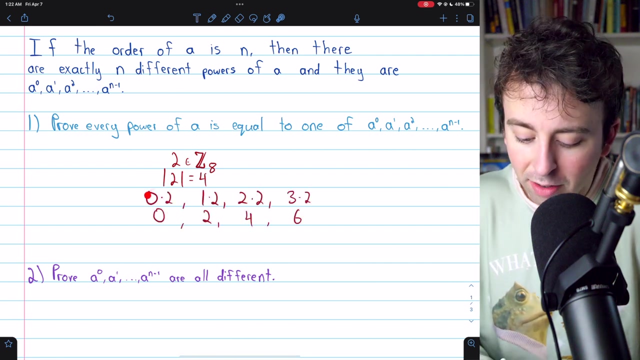 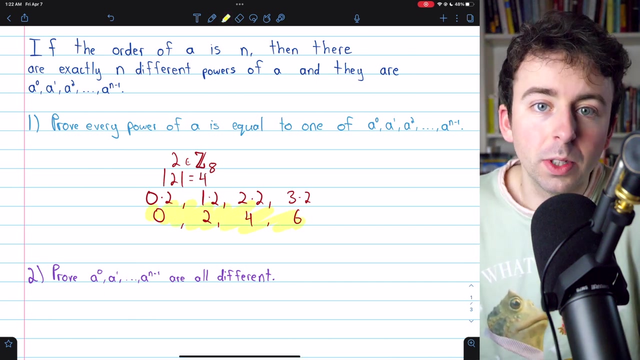 A is an element of the additive group of integers mod 8. So we're going to use additive notation rather than the multiplicative notation that we use to state the theorem. In this group, the order of 2 is equal to 4. And I'll leave a link in the description to my lesson introducing the order of group elements if you need a recap. Now, stating this result in additive terms is to say that since the order of 2 in this group is 4, the first four multiples of 2, 0 times 2 up through 3 times 2, will be a complete list of the multiples of 2. And that looks like this. These are the first four multiples of 2, and it's a complete list. If you look at higher multiples of 2, like 4 times 2 or 5 times 2, etc., they will all be elements of this list. This is a complete list of the multiples of 2. All right, so with that example done, let's jump into our proof. 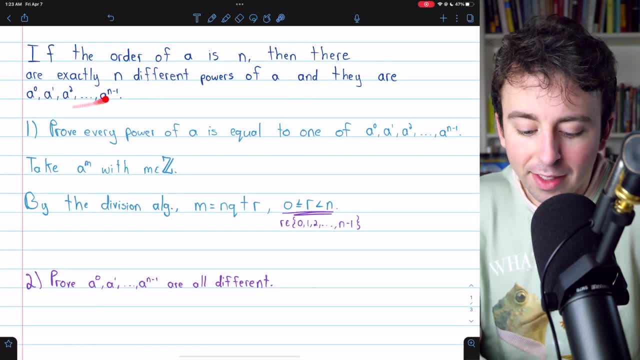 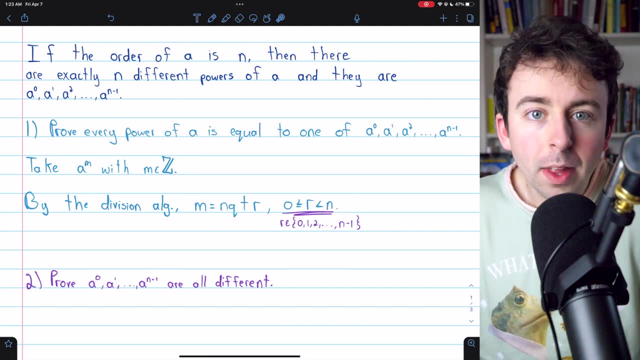 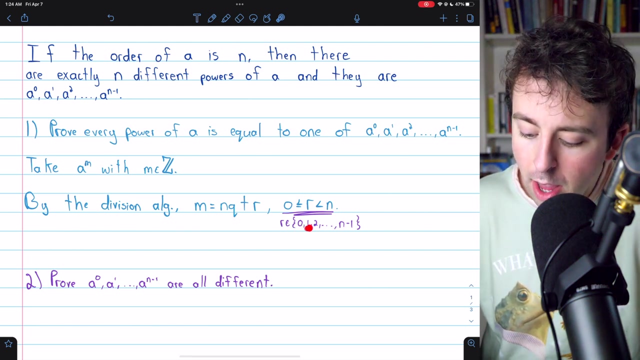 Since we want to prove that every power of a is in this list, we'll begin with an arbitrary power of a, say a to the m, where m is some integer. Then, by the division algorithm, we can divide m by the order of a, which is n. And so we have that m is equal to a's order n times some quotient q plus some remainder r, which must be between 0 and n. I'll leave a link in the description to my lesson going over the division algorithm. If you need a recap, it's a critical detail that the remainder here is at least 0 and less than n. That is a fact of the division algorithm. And in this context, it means that r could range anywhere from 0 up to n minus 1, 1 less than the order of the element a. Those values, of course, are the different powers of a that we have in our list. And that's going to be useful. Since m is equal to nq plus r by the division algorithm, we can divide m by the order of a, which is n minus 1. 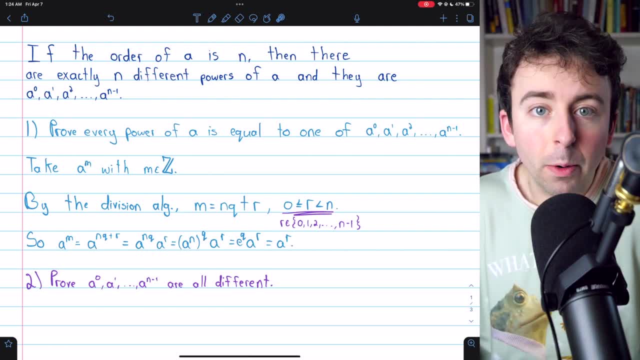 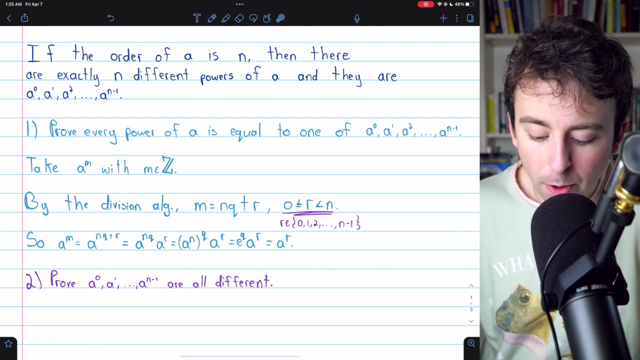 We have that a to the m, our arbitrary power of a, is equal to a to the nq plus r. But then, applying some exponent laws, that's equal to a to the nq times a to the r, which is equal to a to the n to the power of q times a to the r. But recall, n is the order of a. So a to the n is just the identity, which we'll call e. And so a to the n to the q, is just e to the q. So this is e to the q times a to the r. But the identity raised to any power is just the identity. And so we have that this is equal to a to the r. But remember, r is some number in this set. It's between 0 and n minus 1, which means we've taken an arbitrary power of a 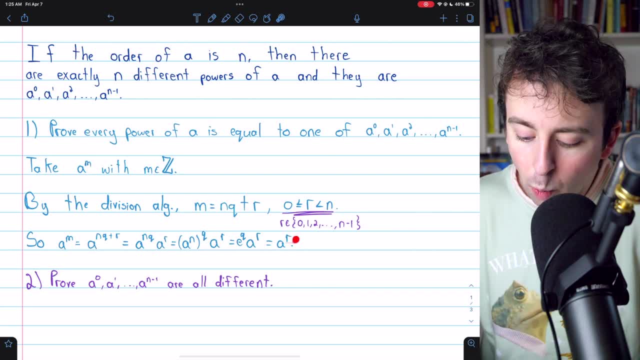 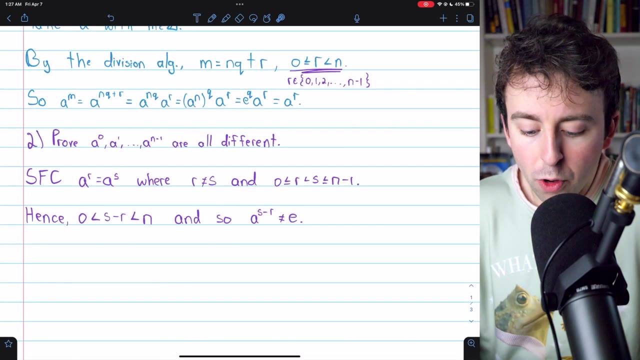 and shown that it's equal to a power of a where the power r is from 0 to n minus 1, meaning that we have a power of a that is equal to a power of a that is equal to a power of a that is equal to a to the m is in fact in this list from a to the 0 to a to the n minus 1. And that completes the first part of the proof. Now we'll prove that all the powers of a in this list 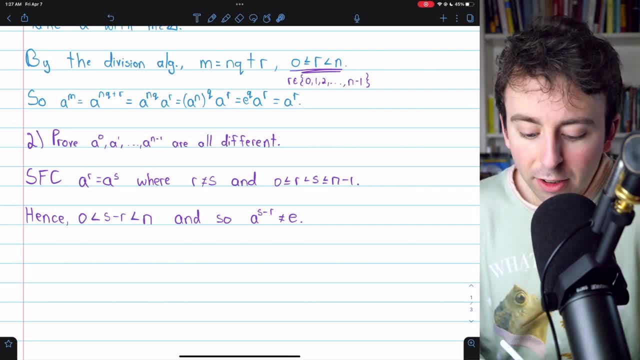 are different. And we'll do this by contradiction. So suppose for contradiction, we have two powers of a, a to the r and a to the s, where r and s are not equal, but the powers of a here are in fact equal. a to the r is equal to a to the s. Of course, r and s we will restrict between 0 and n minus 1 because we're saying that we're taking two powers 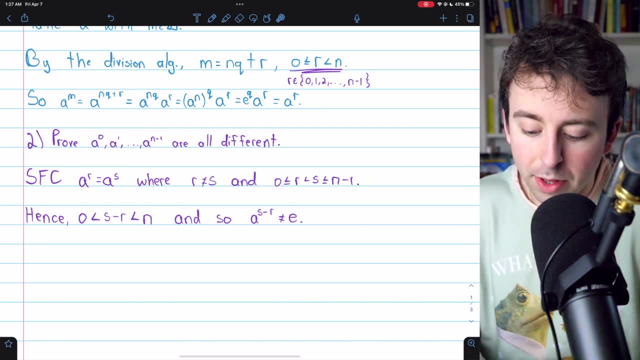 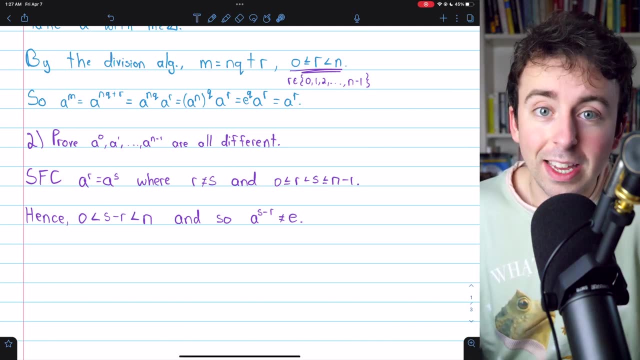 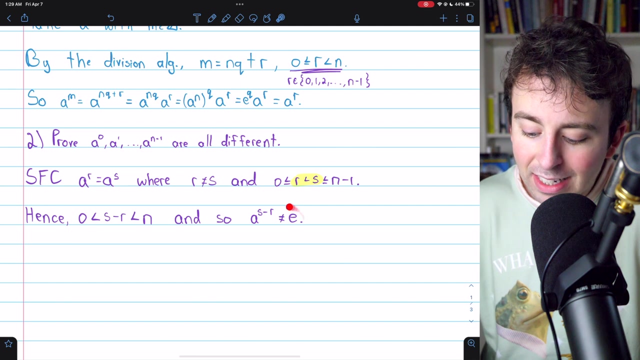 from this list that actually have the same value, even though the exponents are different. And it must be the case, since r and s are distinct, that one is bigger than the other. Let's just say that r is less than s. Then we could subtract r from both sides of this inequality. If r is less than s, then 0 must be less than s minus r. But of course, if s is less than or equal to n minus 1, then once we subtract r from it, that would still be less than or equal to n minus 1, which also means certainly it's less than the bigger number, n. And n is really more important here, so we'll write it like that. Again, we just took this statement that r is less than s, subtract r from both sides, so 0 is less than s minus r, and all of this would still then be less than or equal to n minus 1, which implies it's also less than n minus 1. And then this means that a to the s minus r mustn't equal the identity. That's because s minus r isn't 0, and n is the order of a, which by definition means it's the smallest positive integer, such that a to that integer is the identity. So if we have a positive integer, s minus r, that is less, that is smaller than n, it cannot be that a to that power equals the identity. That's just a consequence of the definition of order. This is going to be our contradiction, because we know that a to the 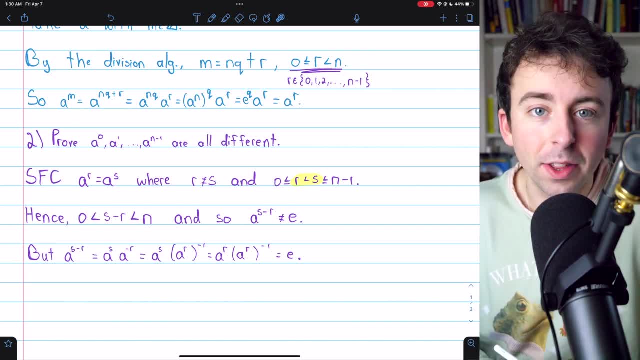 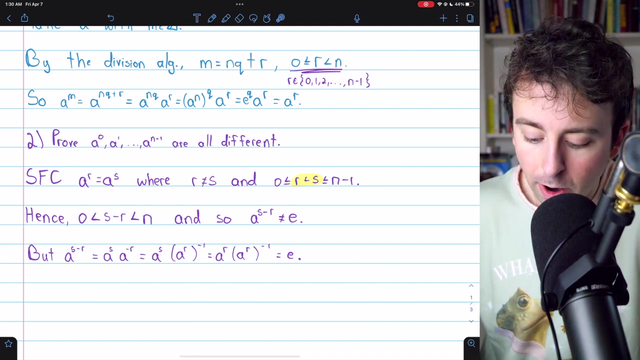 s minus r, this positive integer that's smaller than the order of a, a to the s minus r, by some exponent laws, is equal to a to the s times a to the minus r, which is equal to a to the s times a to the r inverse. But remember, we assume that a to the s minus r is less than or equal to n times a to the s minus r. So we could replace a to the s here with a to the r. So a to the s, a to the r inverse is equal to a to the r, a to the r inverse, which by definition of an inverse element is equal to the identity. There's our contradiction. We showed that a to the s minus r 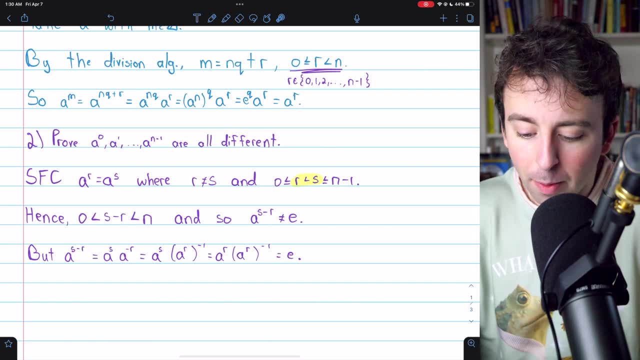 mustn't equal the identity. But then by our contradiction assumption, a to the s minus r is the identity.